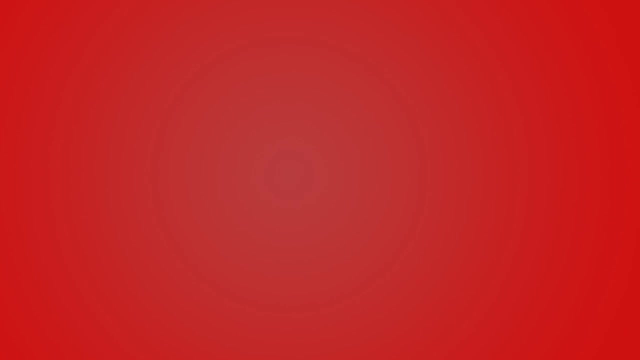 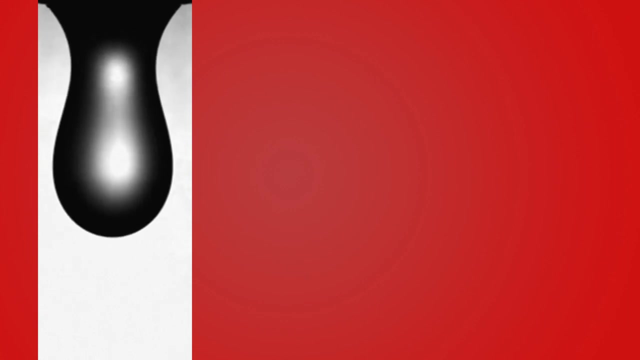 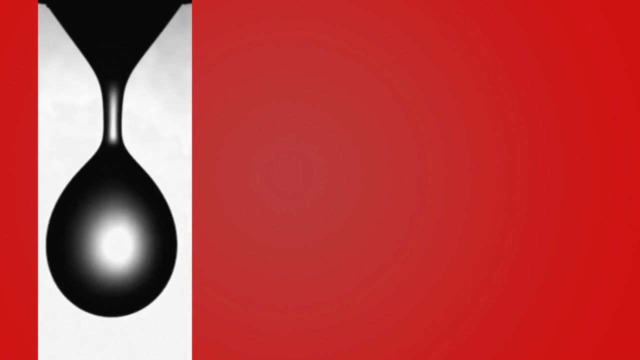 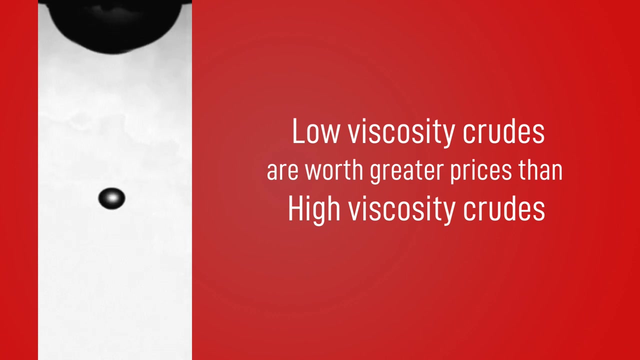 sweet. As for oil's viscosity, the lower the viscosity of an oil, the higher the fraction of short-chain liquid hydrocarbons in the oil. Ext Ath Lynx ℕ High Test weather ratio: 10 BE. Si Tra 로 7 ℕ ℇ. 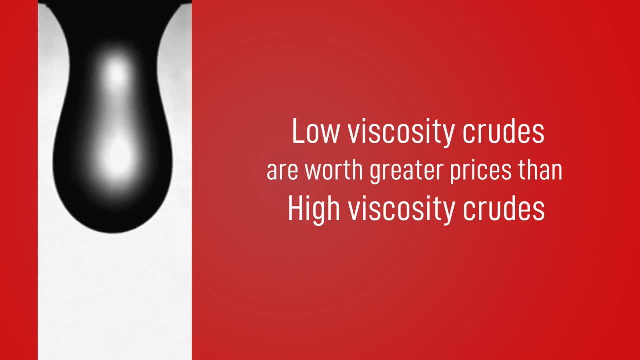 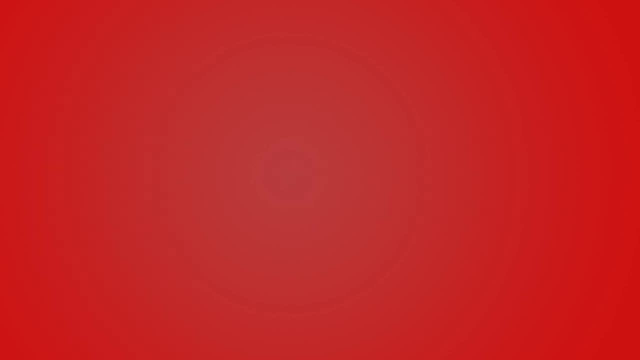 ℆ ℇ � Transform into lead ℇ ℛ ℆ ℊ ℕ ℆ Among the different types of crude oils are a special set of benchmark crudes. A unique set of benchmark crudes is among the several sorts of crude oils. 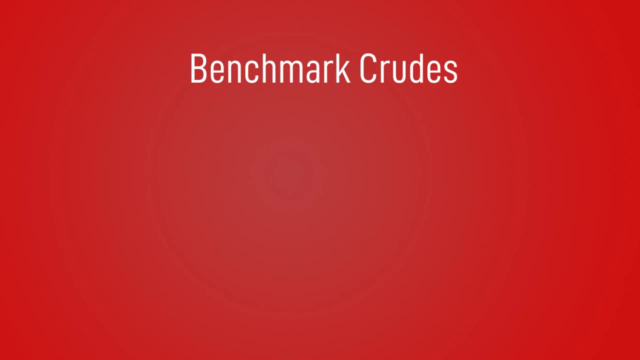 These benchmarks are crudes with well-defined hydrocarbon, sulfur and viscosity characteristics. West Texas Intermediate Crude, or WTI, is the most well-known of the benchmarks, And then there is Brent Crude, which originates from the North Sea. Both WTI and Brent are light, sweet crudes. 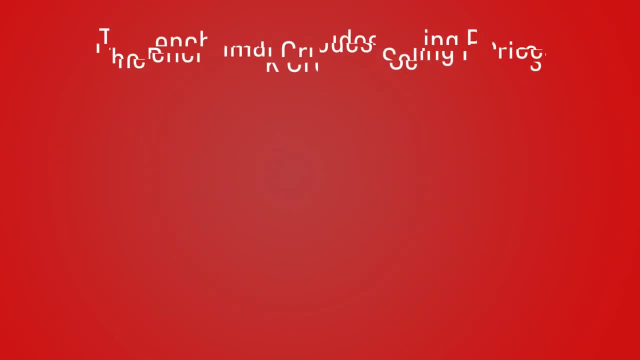 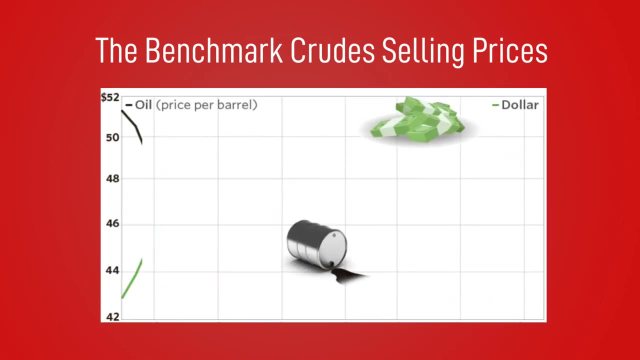 The benchmark crudes selling prices are frequently publicized. This is due to the fact that the prices serve as standards for determining the daily prices of practically all other crudes in the world. Leaving aside other price influencing factors, the sale price of crude oil will differ from. 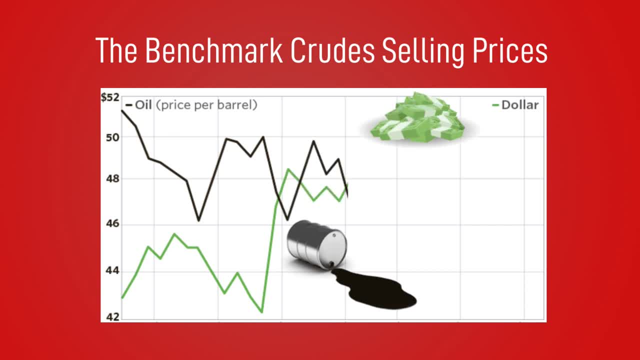 the market price of a benchmark crude by a quantity that reflects the particular price, In particular crude's hydrocarbon content, sulfur content and viscosity in comparison to the benchmark crude's specifications. As a result, a crude produced with a greater sulfur concentration and viscosity than WTI. 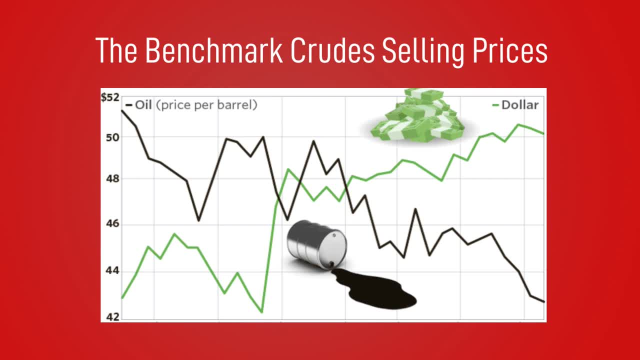 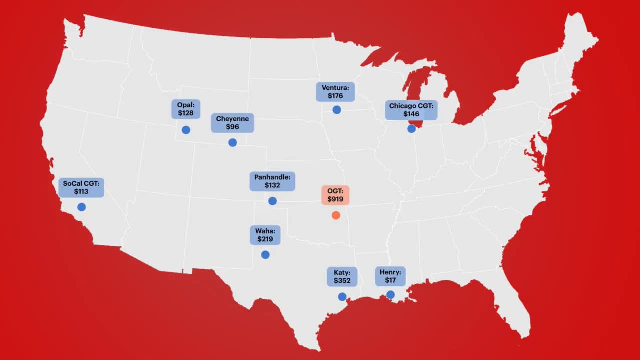 will typically be priced at a reasonable discount to WTI. There are benchmark prices for natural gas, in the same way that there are benchmark prices for oil. In this case, the benchmark pricing are for oil. The benchmark prices are for processed natural gas delivered to a specific site. 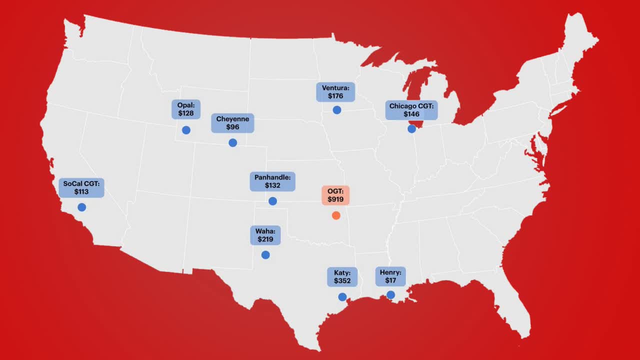 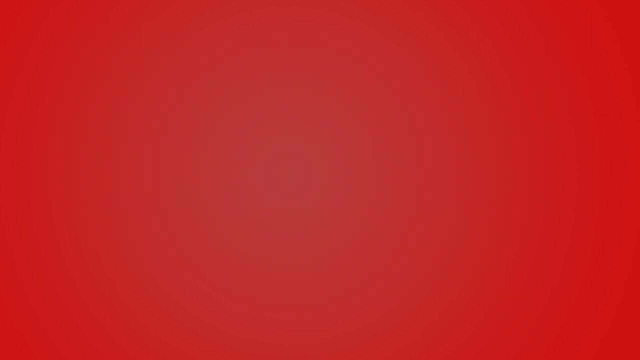 These are commonly referred to as natural gas hubs. The price of processed gas sold elsewhere is frequently changed in relation to the price of natural gas at the benchmark hub, dependent on the distance between the hub and the alternative sale point. The price of oil, natural gas and petroleum products is not solely determined by the cost. 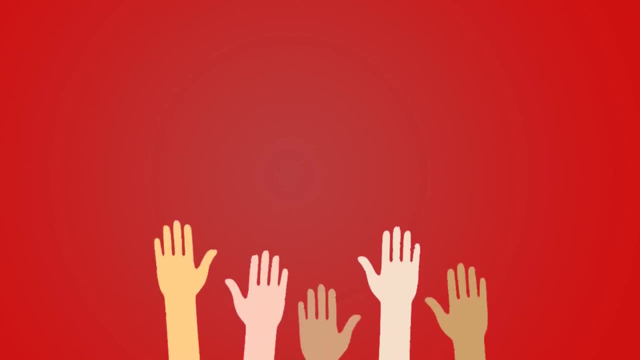 of producing these fuels. The price of oil, natural gas and petroleum products is not solely determined by the cost of producing these fuels. It is also affected by the demand for fuels. Oil prices have climbed over the last several decades as we have had to spend ever-increasing 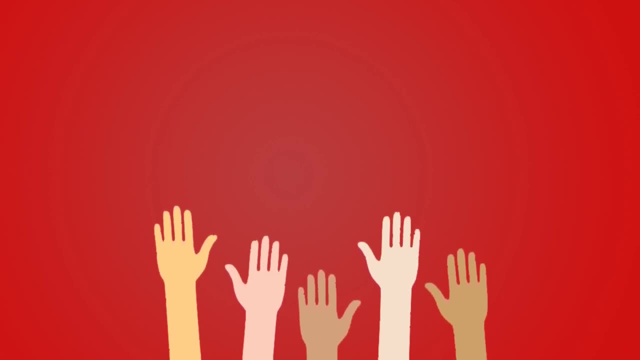 costs in order to produce enough oil to fulfill rising demand. And given that demand appears to be increasing in the future, it's logical to expect oil prices to grow as well. However, looking at past oil prices, it is evident that the price can play a role in. 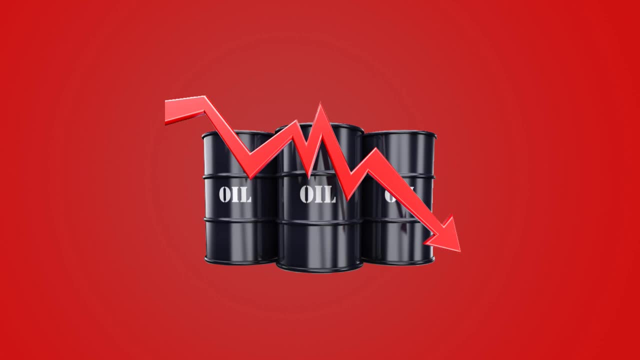 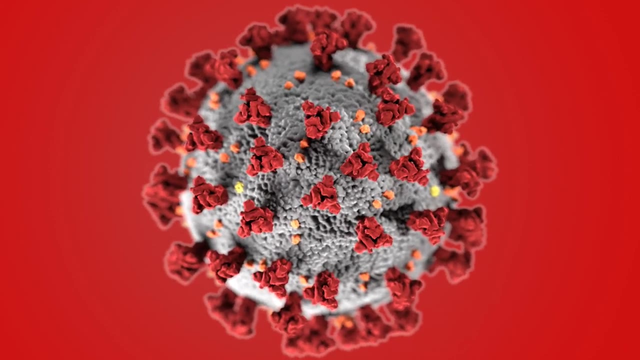 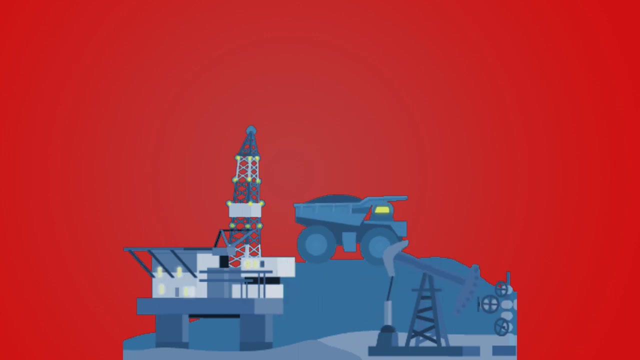 reducing oil prices significantly. There are two possible causes for such falls. One example is a drop in global demand, as seen during the COVID-19 epidemic spread. Another factor that could drive prices to fall is a technological advancement that reduces the cost of producing previously expensive oil reserves. This is what happened from 2013 to 2015, when the cost of horizontal drilling and fracking declined. The oil prices have gone up, allowing these technologies to be employed to obtain previously expensive shale oil, Natural gas and certain distillate fuels such as gasoline, diesel, heating oil and. 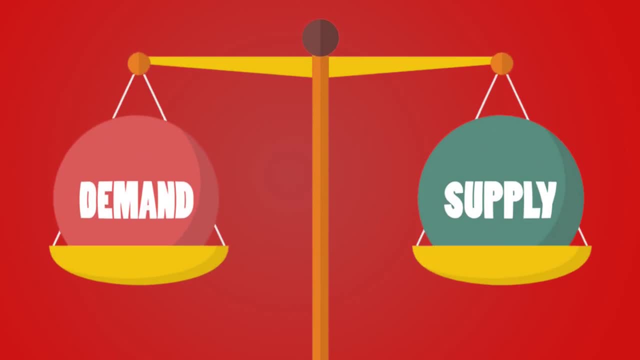 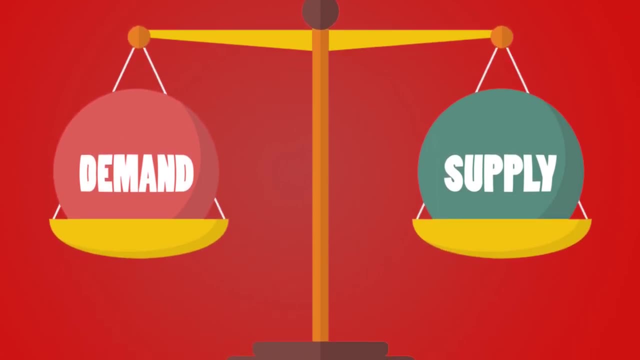 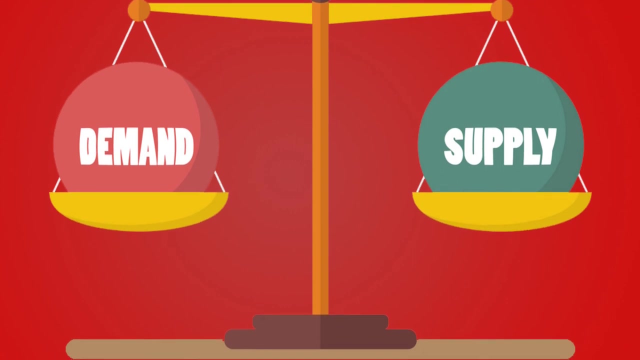 propane undergo large seasonal fluctuations in demand. As a result, supply and costs of these fuels might vary greatly from season to season. Residential and commercial use of natural gas, for example, is predominantly for space heating. Hence natural gas demand in these sectors is highest during the winter months. 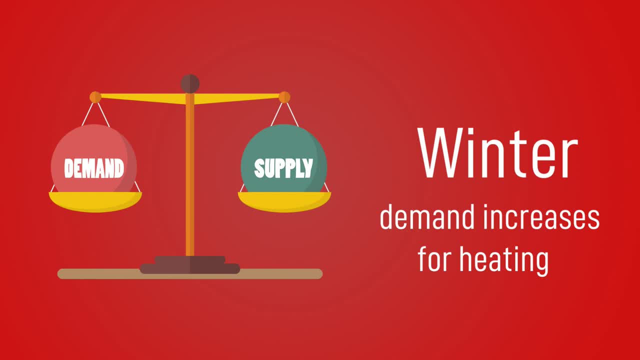 The same is true for heating oil and propane, both of which are used for heating in the home and commercial sectors. During the summer, however, residential and commercial demand switches to increasing air conditioning consumption, Because the increased demand for electricity is mostly provided by natural gas power plants. the electrical sector's demand for natural gas is reduced. This means that the demand for natural gas is reduced. This means that the demand for natural gas is reduced In general. the fuel production is lead by demand for pure gas pumps, such as gasoline and diesel.